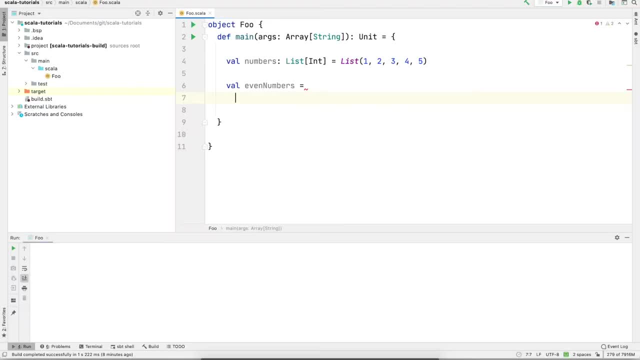 can be different from the input collection. So we take the numbers collection as and then say something like dot map, and then that's how the signature goes. Element is the current element in the iteration on the collection. Then we can say element multiplied by two. So how it works is that it goes through each element and multiplies. 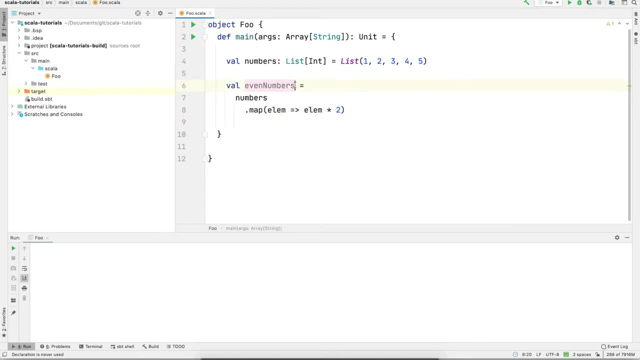 each element with two. so to convert into even numbers We can look at what the type is. So the type is same as the given type with collection of int. but that is not necessary. It depends on the function that we are applying Here. our function is multiply element with two. 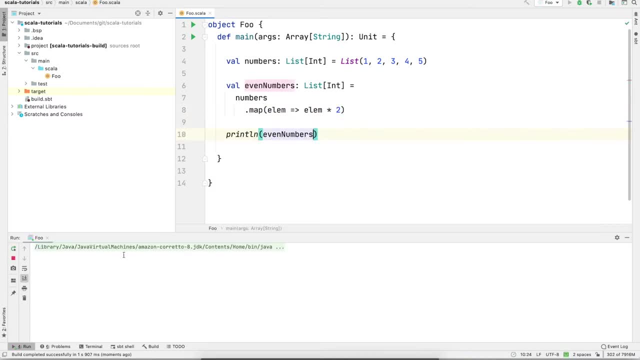 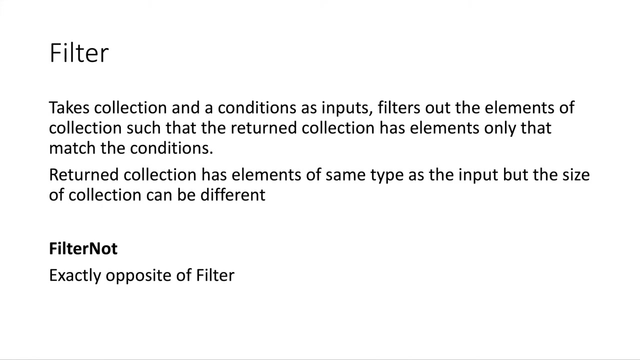 And here you can see we have a list in the result which is has five elements as the input list. Next one is filter. Filter takes a collection and a condition as input. It filters out all the elements of collection in a way that the elements that fulfill the condition provided are kept and 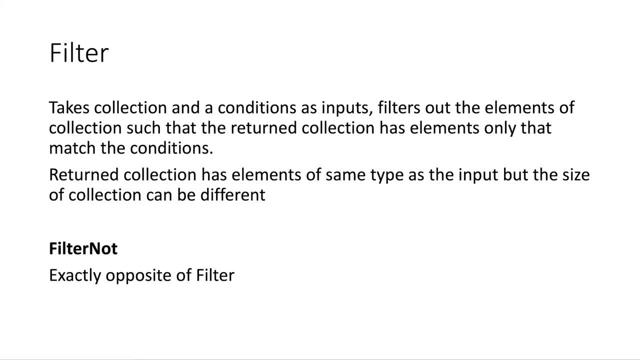 all other elements do not appear in the returned list, which means that the size of the returned collection can be smaller than the input collection, but the type of elements remain the same. Similarly, there is filter not, which is exactly opposite to filter, which means the elements that do not. 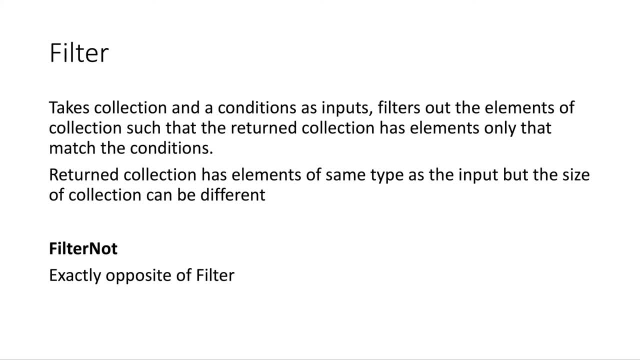 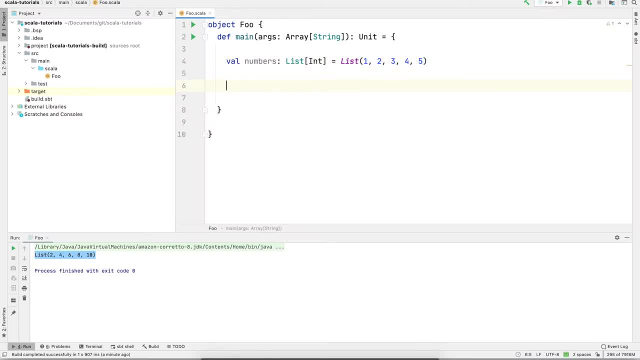 fulfill the provided condition are returned in the returned collection. And in this example we can. we can try to filter out only the even numbers. Take the collection, apply the filter method. take each element and element modulo two equals to zero. So this here is a Boolean condition. 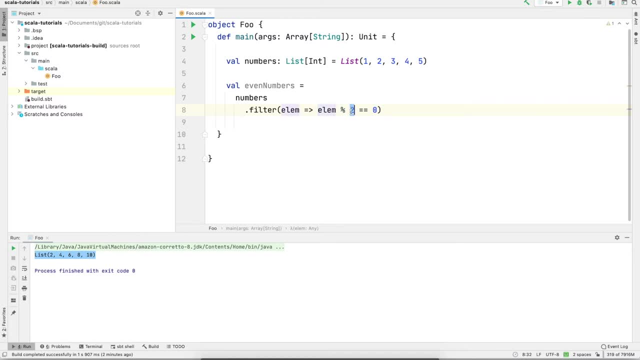 What this means is that if you divide this element by two, its remainder is what I want. So if remainder is zero, then of course it means even number. If you look at the return type, it's the same as the input collection. Here you can see that in this list we get only two even numbers: two and four. Next one is: 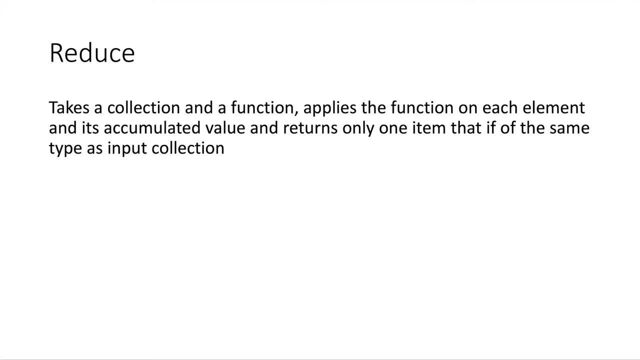 reduce. Reduce takes a collection and a function. It applies the function on each element and its accumulated value. So it basically accumulates values over iteration And the last return is only one item, and that item is of the same type as the input collection. 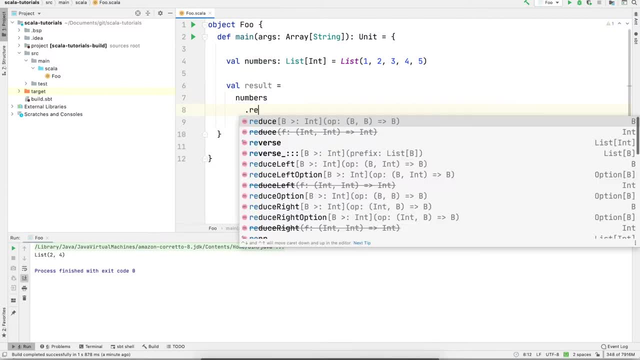 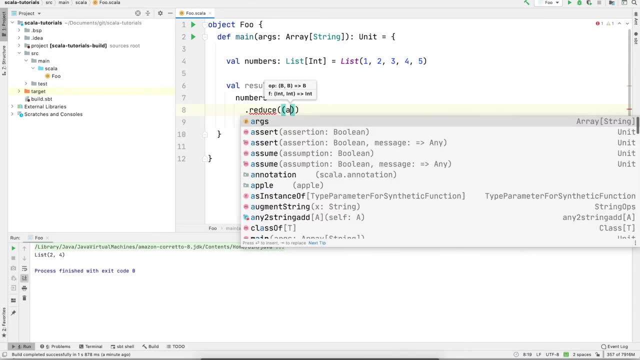 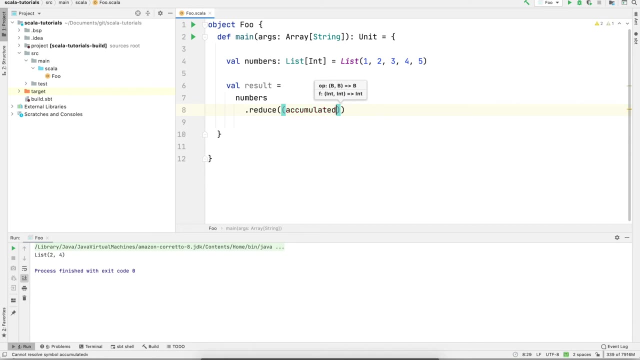 We have our numbers, Try to reduce them, And the signature looks a little bit different because now we have accumulated value with current element in the iteration And what we want to do is, let's say, we want to sum. If you look at the return type, you can see that it's no more list of integers but just one integer. 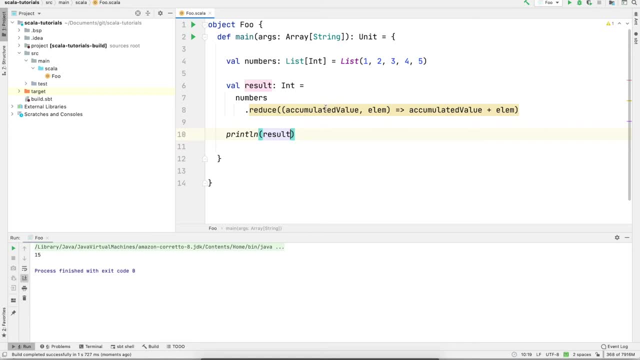 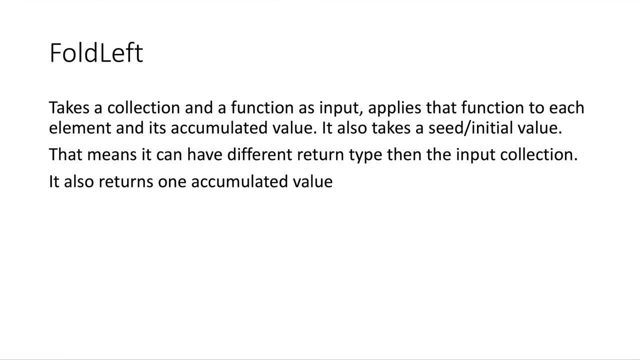 So it's 15.. So basically, how it works is that here it's accumulating the value and each iteration it is adding that accumulated value with the new element. So overall the value is 15.. The next one is fold left. Fold left is quite similar to reduce, except, unlike reduce, it has an additional input parameter, a seed value, the value where to start accumulation with. The second difference is that, unlike reduce, the return type can be different than that of the input list. 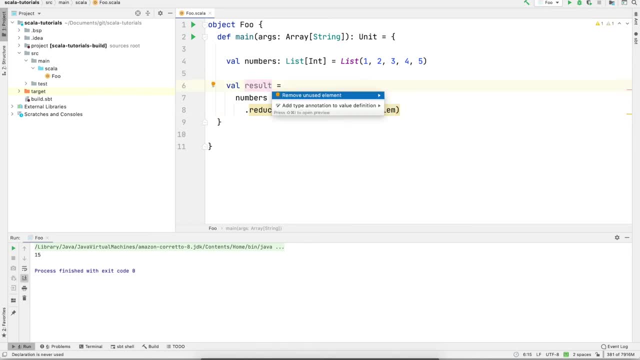 Here is our example of reduce. The return type here is int, which is the same as the return type of the collection. But let's assume our function here instead of addition is something that can change the result type. For example, if we want to do a divide and we don't want to have an int result, but we want to have more exact result, more precise result, let's say, for example, double. 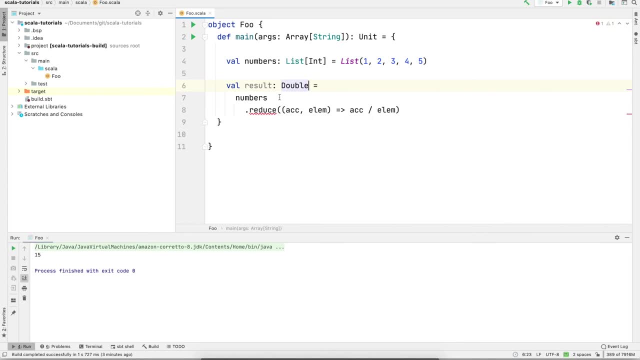 Now, reduce won't work because the types of incoming collection is int and the resultant expected is double. So let's try how this can be done through fold left. Additionally, we have another parameter list that we need to give, which is the seed value. We can do seed value with one. 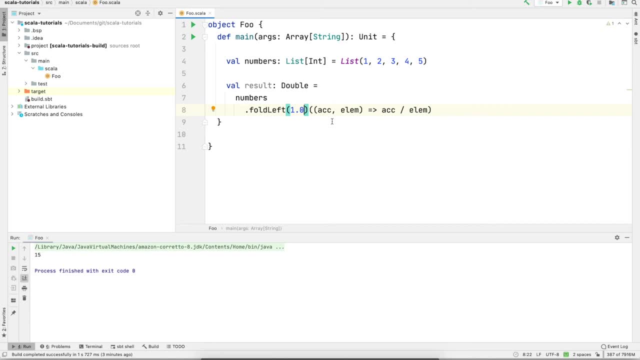 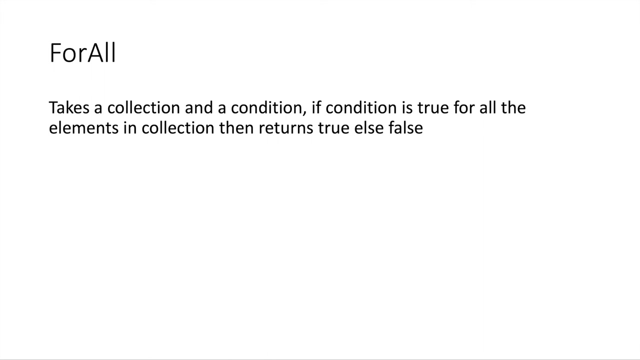 So what does this mean? is that we are going to start with one and keep It dividing with the element in each iteration, accumulating the result. The next one is for all. So for all takes a collection and a condition, a Boolean condition. 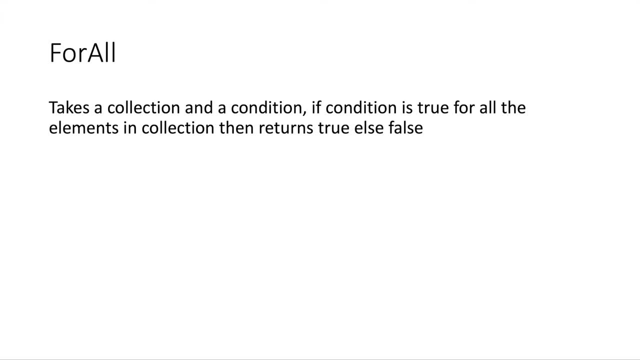 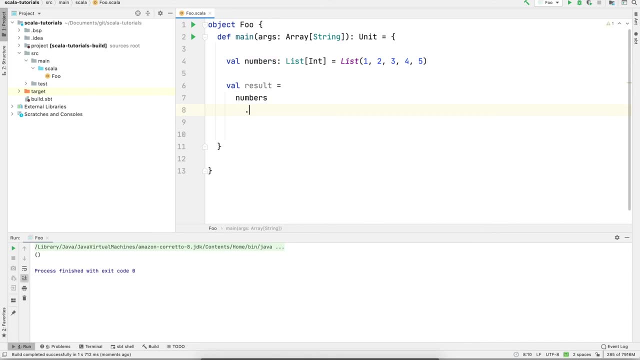 If the condition is true for all the elements in the collection, then it returns true. We can basically check if all the elements, If all the elements in this collection are even numbers. so we take element if divided by two as a remainder zero. 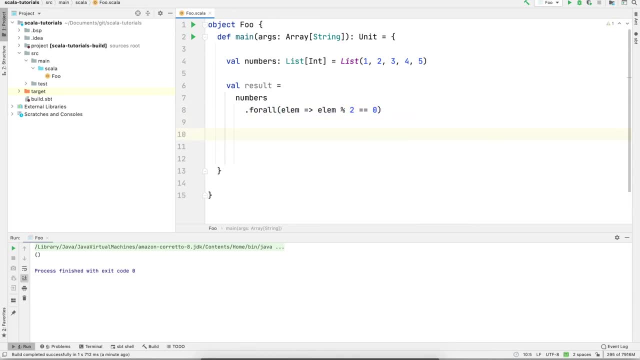 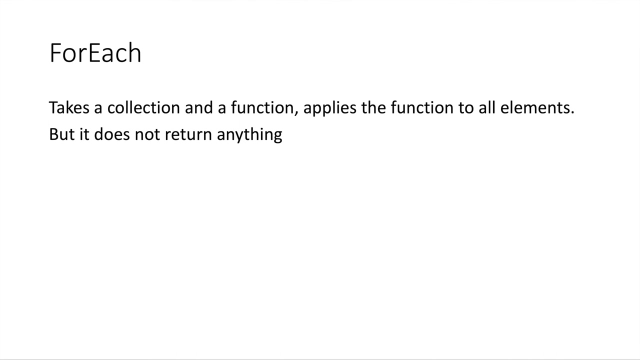 Then it should be an even number. It's false because we have few odd numbers in here. Next one is for each. So for each takes a collection and a function and it applies to all the elements in the function. It sounds similar to map, but it really isn't. 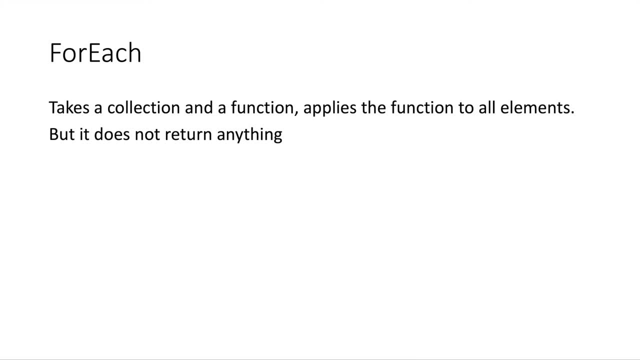 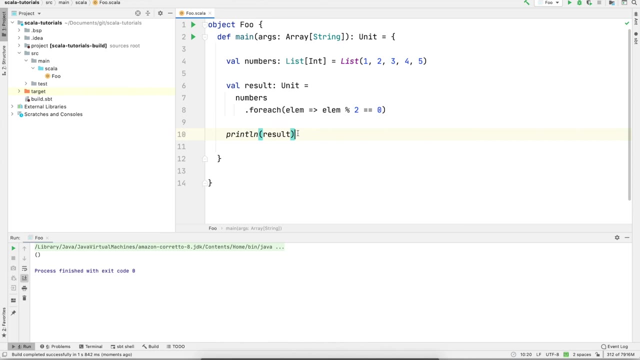 In map you always have a return collection, but in for each you do not return anything. You apply the function but you do not collect the value of that application. A very common example of using for each. The reason is that instead of printing the whole collection here,